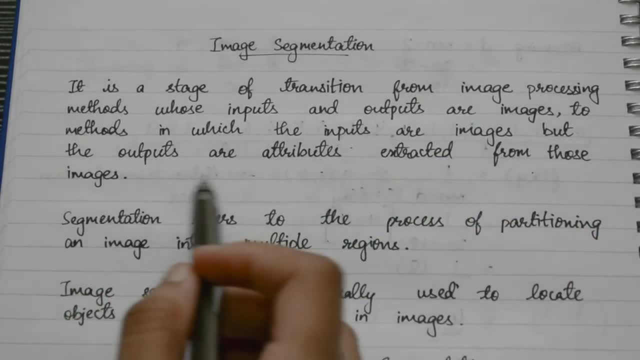 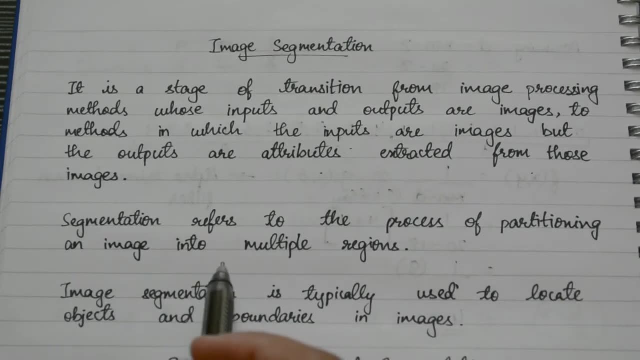 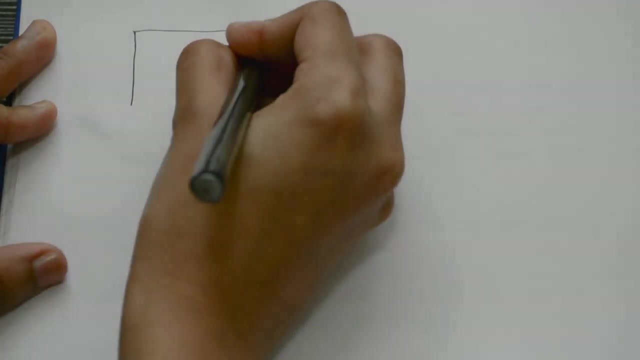 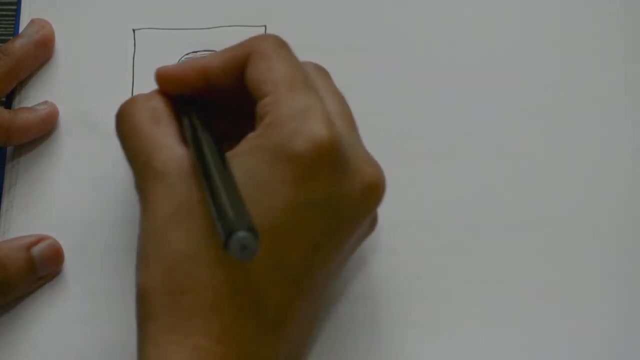 to methods in which the inputs are images but the outputs are attributes extracted from those images. Now, segmentation refers to the process of partitioning an image into multiple regions. So suppose if we have an image here and in this particular region, it is high intensity- okay, which means that all the pixels in this region are of high intensity values, okay. 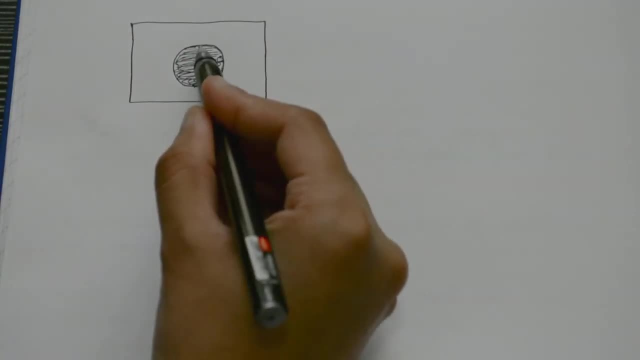 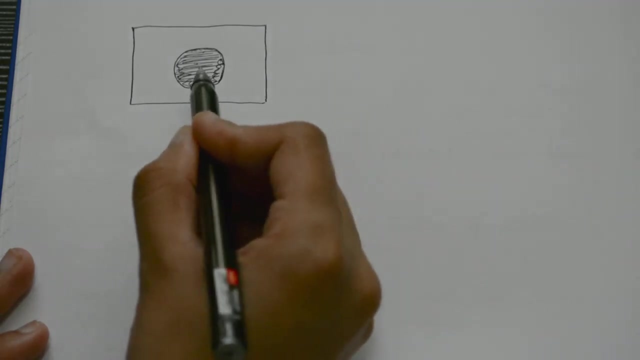 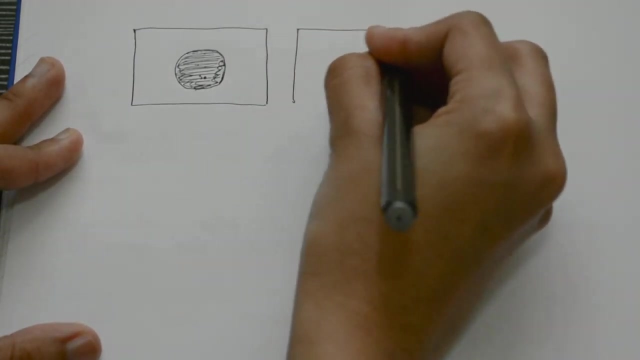 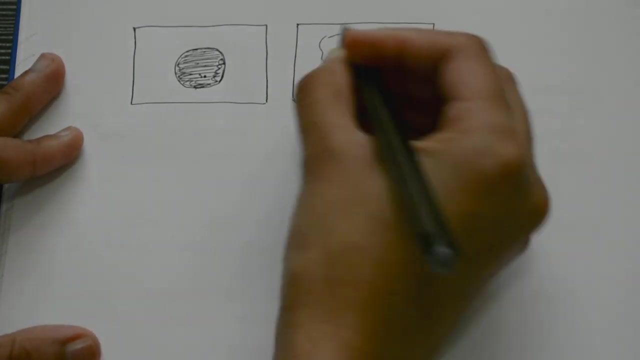 So what does image segmentation do? It identifies, it locates these abrupt changes in intensity values and it identifies this as an object: okay, it detects this object. Similarly, if we have another image here and in these particular regions, okay, all of these have similar intensity values, which means that all pixels in this 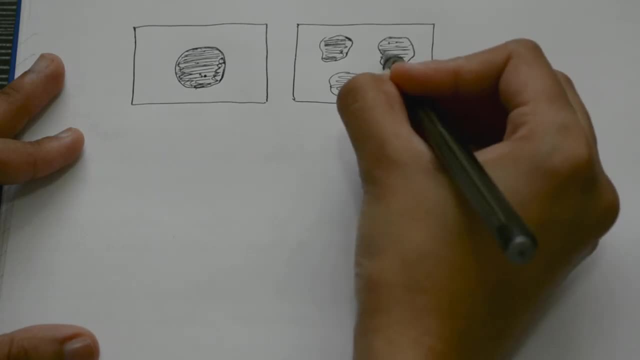 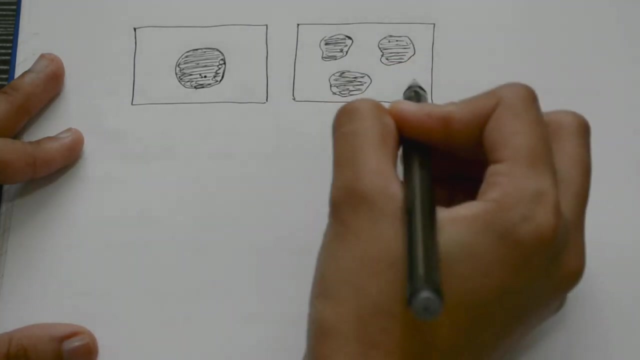 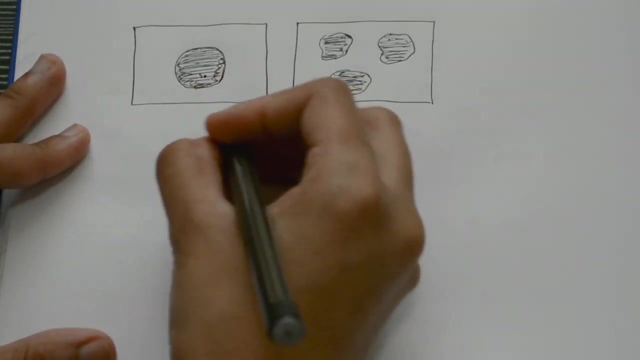 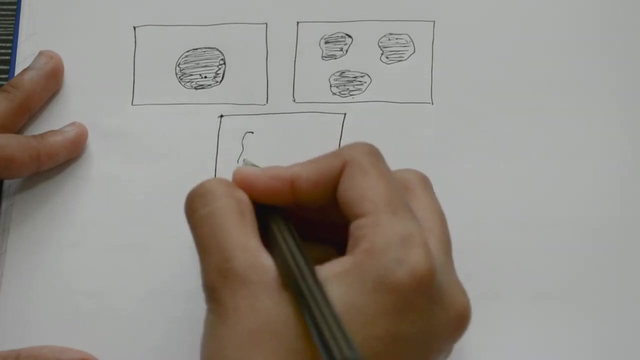 region have similar intensities. All pixels in this region have similar intensities. So, based on these similar intensity values, it segments this image, which means that it splits this image, this entire image, into different regions. okay. Similarly, if we have another image here, okay, and there is an object in this, but the boundaries are not complete. So 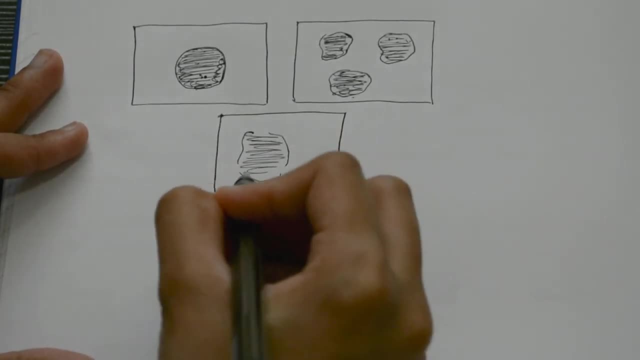 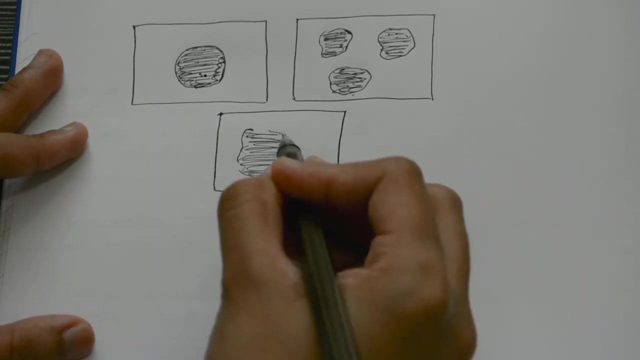 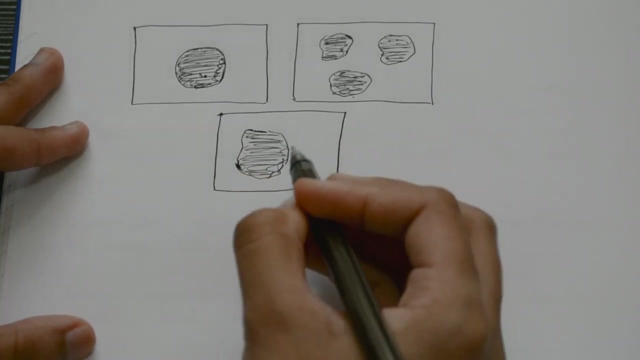 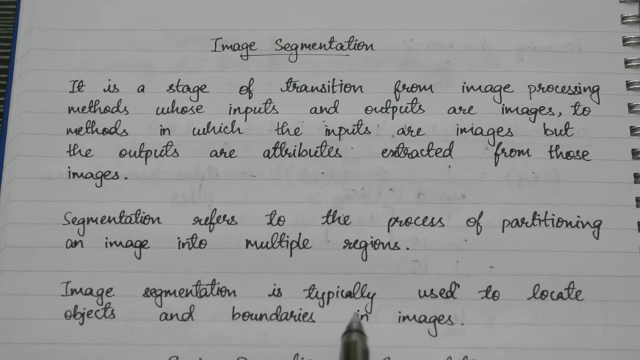 image segmentation helps in boundary detection. okay, It checks for the intensity values, all of these, all of the intensity values and this have similar values. okay, So, based on that, it does boundary detection, okay, line detection or edge detection. So all of those were applications of image segmentation. So image segmentation is typically used to locate objects and boundaries. 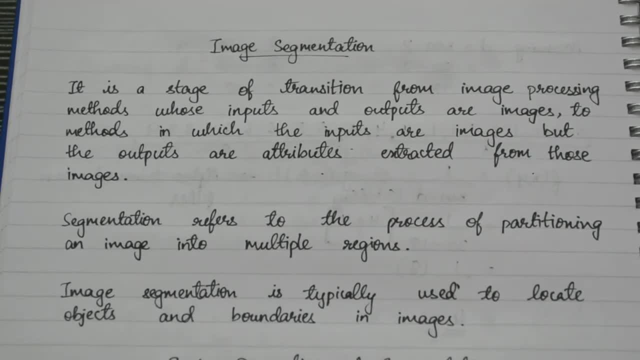 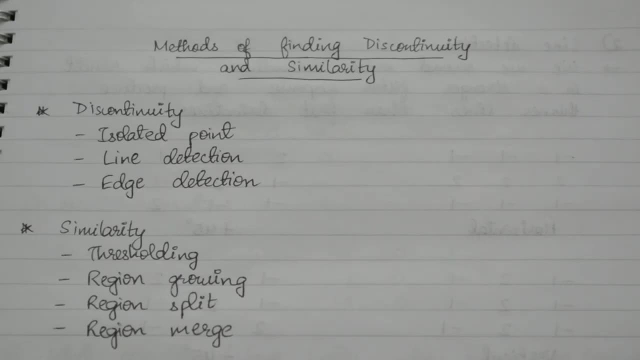 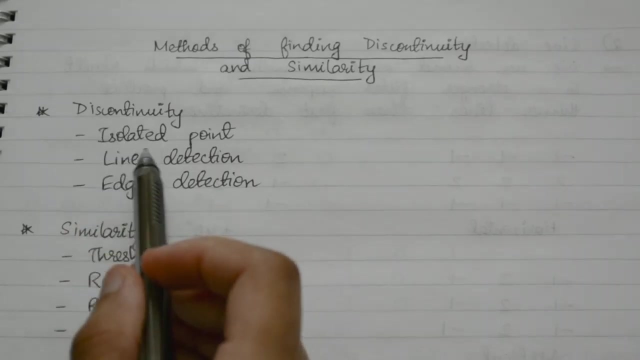 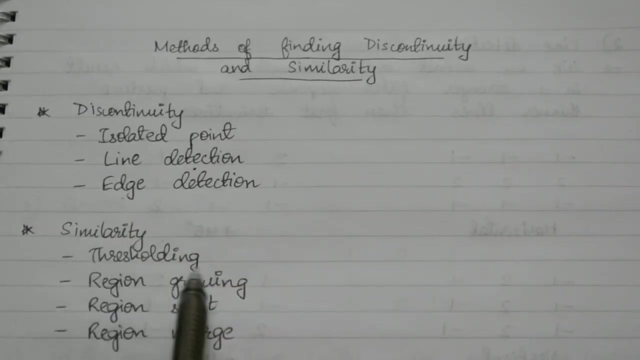 in images: Methods for finding discontinuity and similarity. Now, there are different methods for finding the discontinuity in an image and those different methods are isolated point line detection and edge detection. And for similarity, the methods are thresholding, region growing, region splitting and region merging. okay, I will explain this in detail and we will 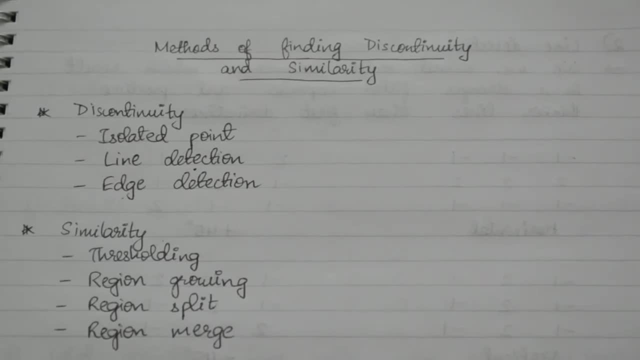 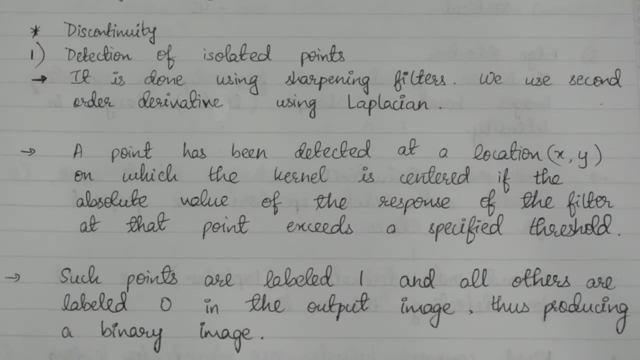 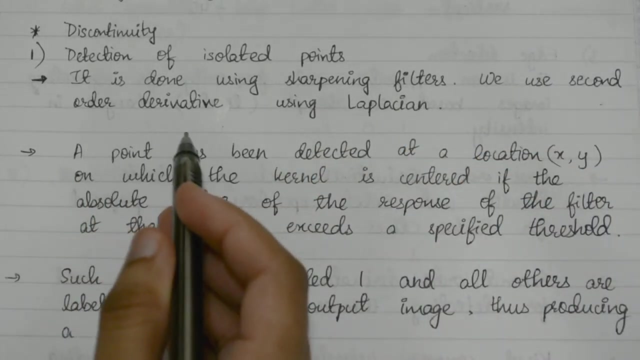 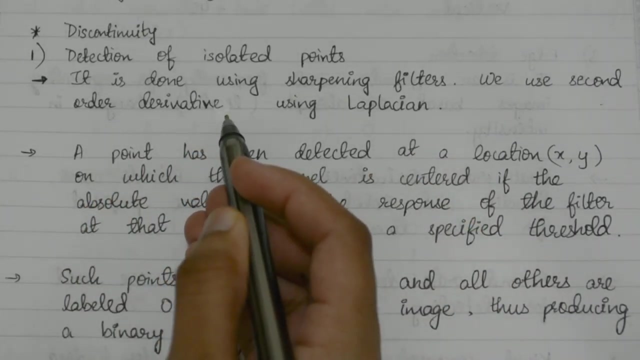 also do some more details in the next video. Now let's look at point detection, which comes under discontinuity. Point detection is done by using sharpening filters. We use second order derivative using laplacian. okay, So we have studied this earlier. If you haven't watched the previous videos yet, then kindly. 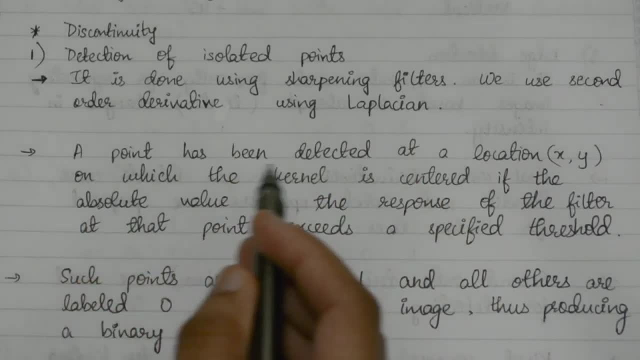 do so before watching this one. Now, a point has been detected at the location of point. The point has been detected at the location xy, on which the kernel is centered, if the absolute value of the response of the filter at that point exceeds a specified threshold. 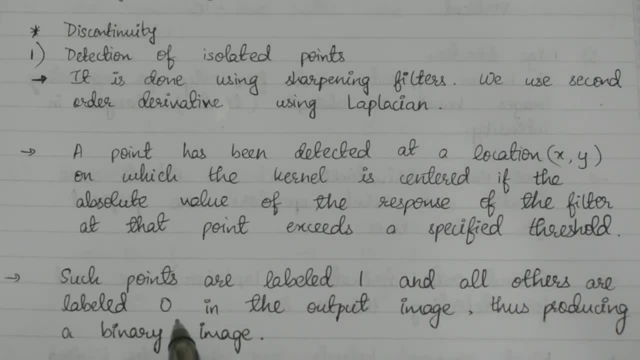 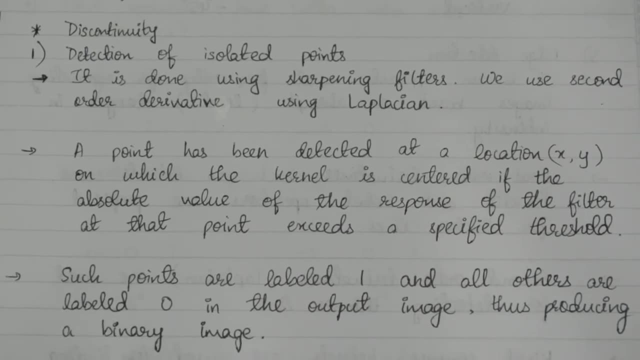 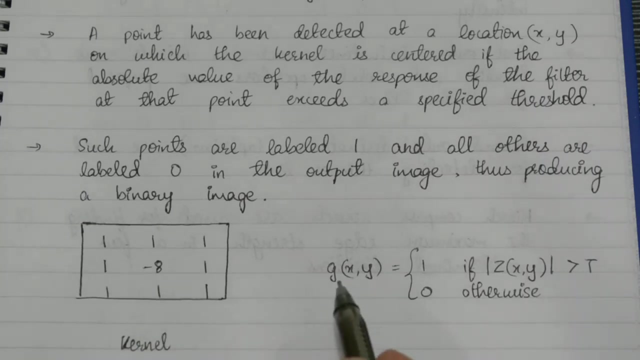 Such points are labelled 1 and all others are labelled 0 in the output image, thus producing a binary image. Now you can see, here we have the kernel for point detection, and the function for point detection is: g of xy is equal to 1 if the absolute value of z of xy is greater. 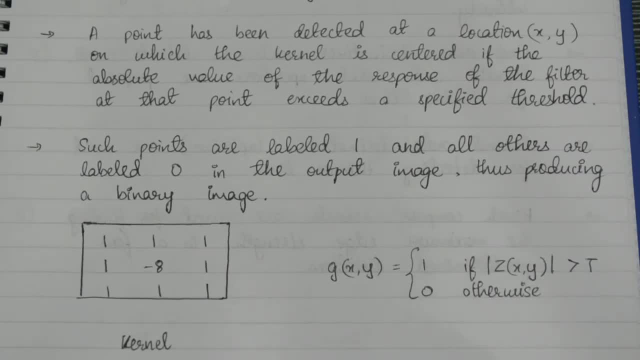 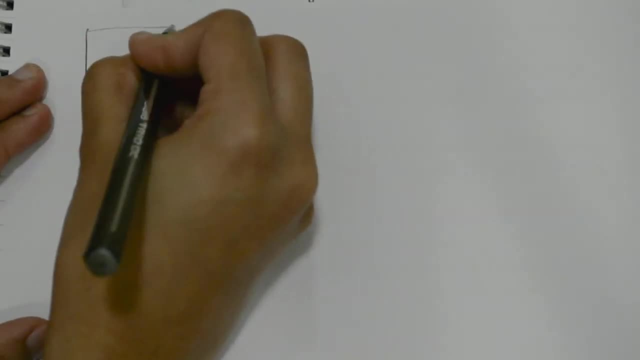 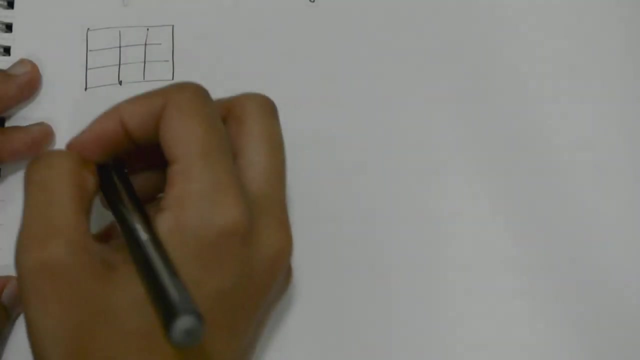 than t and it is 0 otherwise. Now, what does all of this mean? Suppose, if we have our input image- okay, a 3 by 3 input image- what will be our first step? We do padding of some sort, okay, So we will get our padded image. 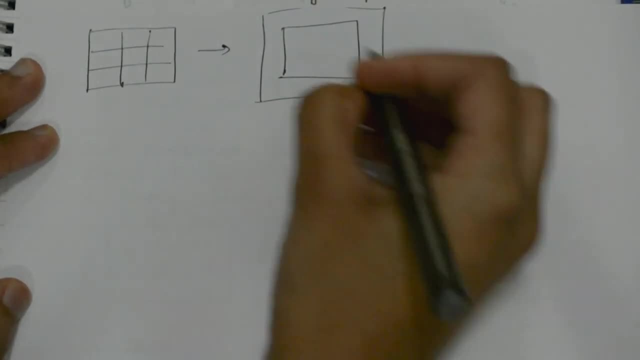 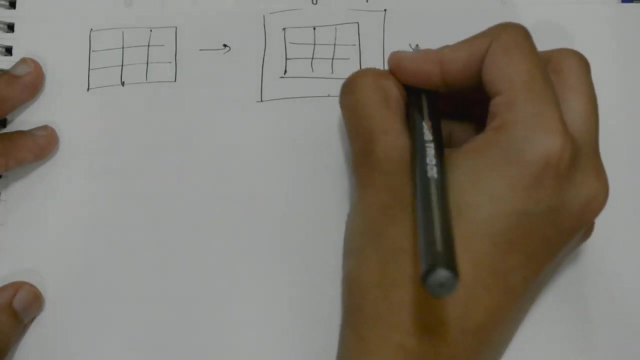 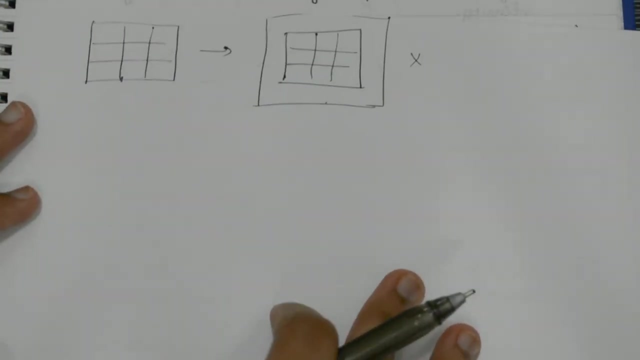 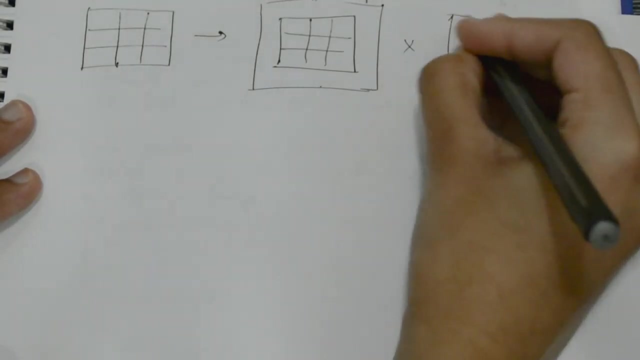 We can use any sort of padding, 0 padding, pixel replication, any sort of padding, and once we get the result from it, we will use the mask. okay, So this mask for point detection, we will apply the same mask. okay, We will apply this mask on the image and the result. 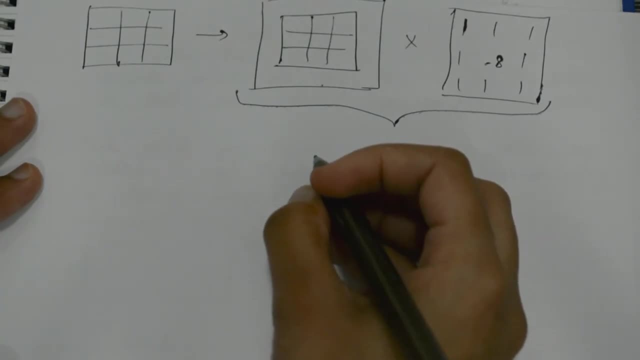 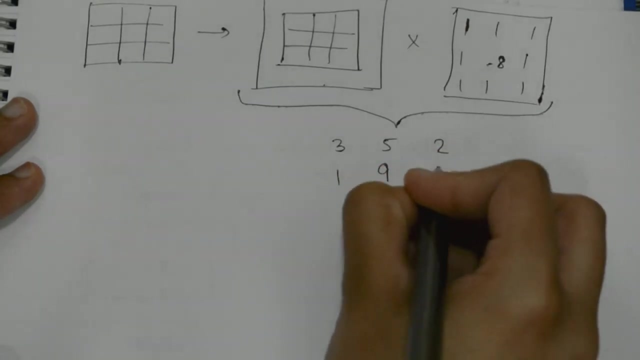 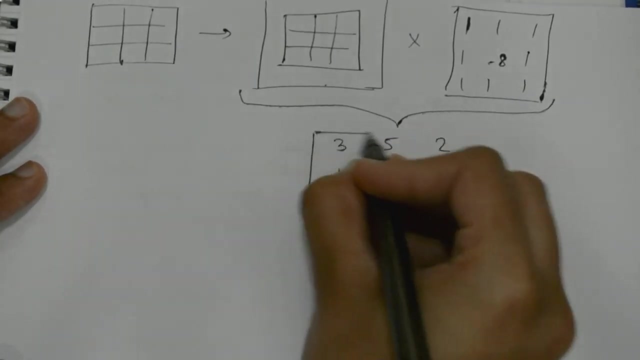 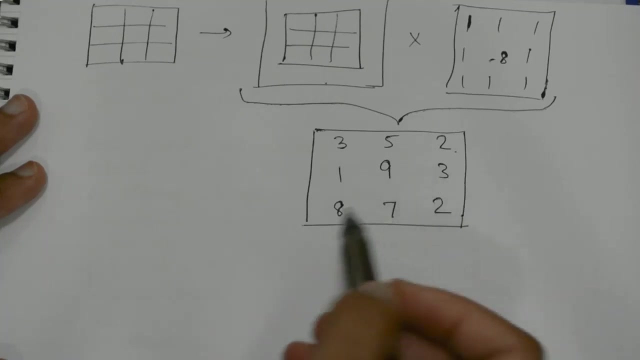 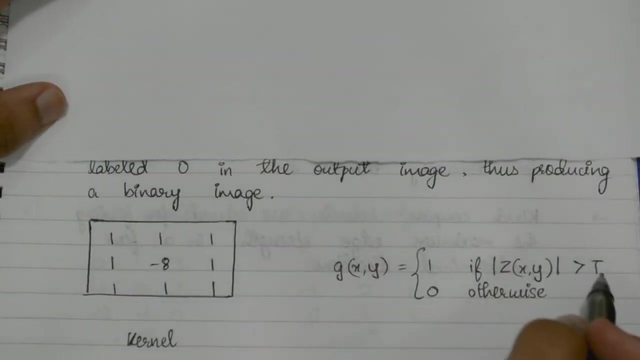 which we get from that. Suppose the result is 352913872. okay, Suppose this is our result, then what we will do is we will check each of these pixel values with the threshold value. Now, the threshold value will be given in the question, suppose, and that is known as t. Okay, So this is our result. 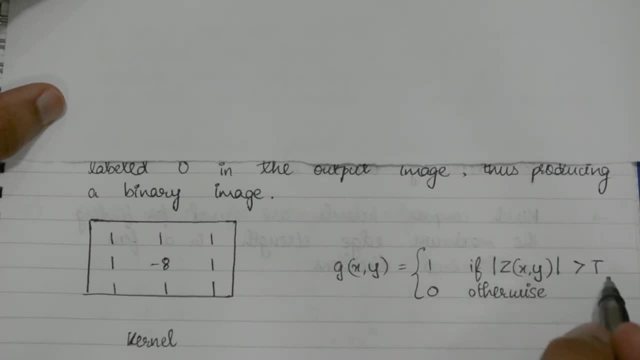 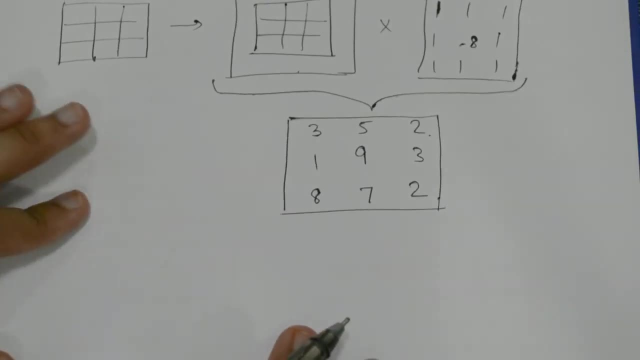 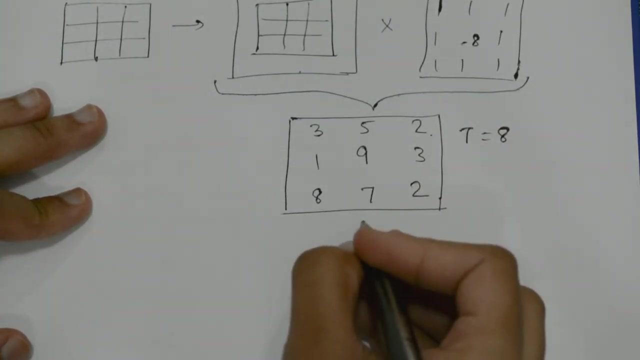 t is the threshold value We have to check. If it is greater than t, then the value would be 1 and it would be 0. otherwise, Suppose in this example t is equal to 8.. So what will be the output of this? First we check with 3.. 3 is less than 8, right? So we put. 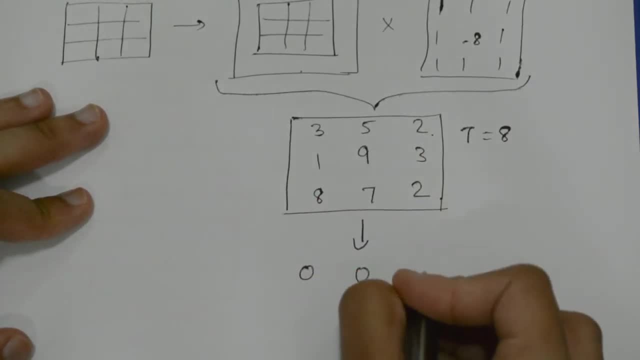 0.. 5 is less than 8,. 0.. 2 is less than 8, less than 8.. Now, 9 is greater than 8, so we put 1.. Here we put 0.. 8 is less than or equal to. Here, if we check, it has to be. 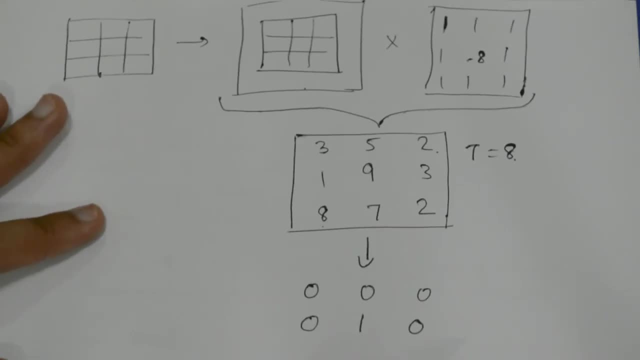 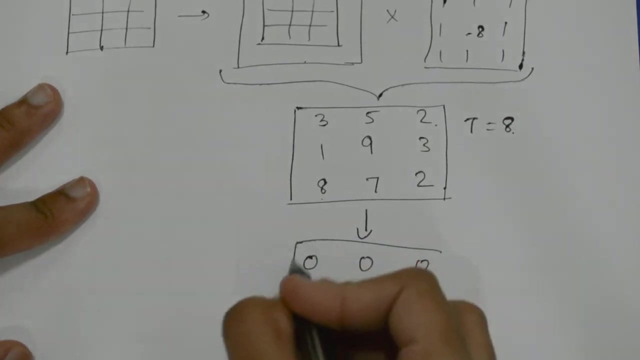 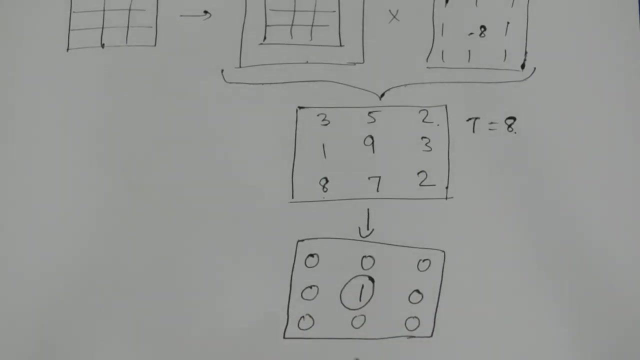 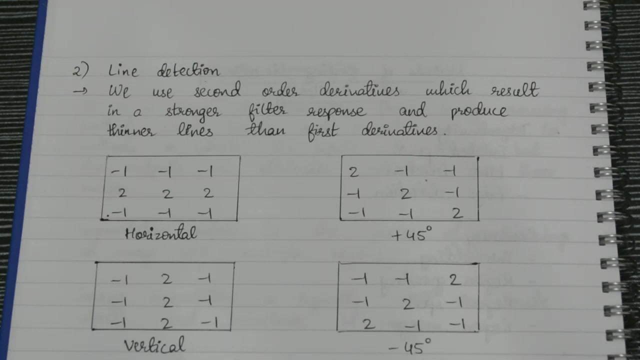 greater than: okay, So here 8 is less than or equal to. It comes in the otherwise category, So 0,, 0 and 0.. So in this way we have to check, We have to detect the point over here. okay, So this is how it is done for point detection. 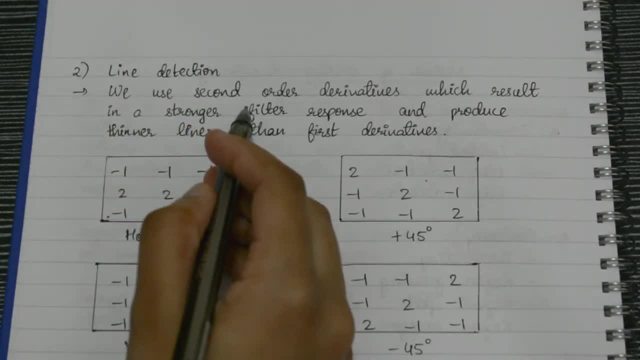 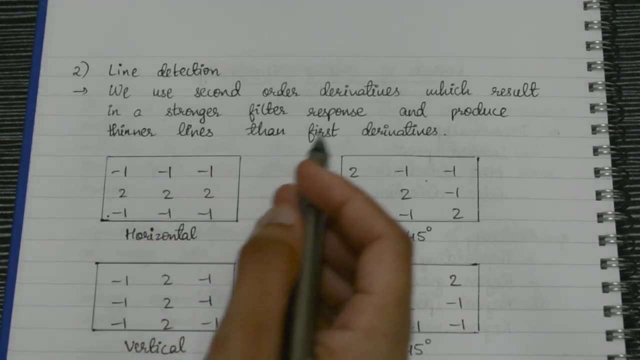 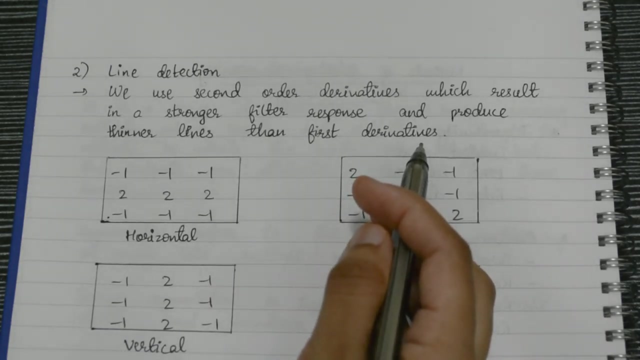 Next we have line detection. We use second order derivatives here again, which result in a stronger filter response and produce thinner lines than first order derivatives. okay. So for thicker lines we use first order derivatives and for thinner lines we use second order derivatives- okay, Which produce a stronger filter response. we use 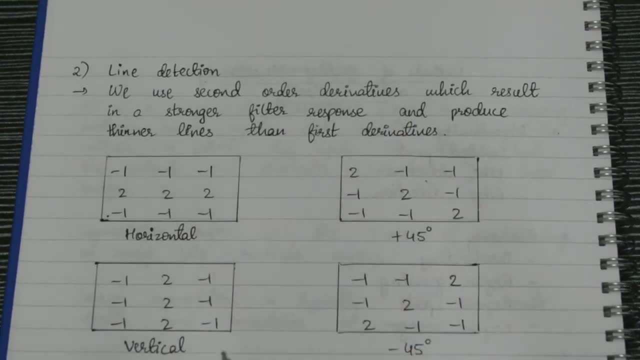 second order, derivatives: okay, The kernels here for horizontal lines, for detection of horizontal lines, is this one, For vertical lines it is this: and if it is any line at a given angle plus 45 degrees, okay, Then we use this. okay, It means, if a horizontal 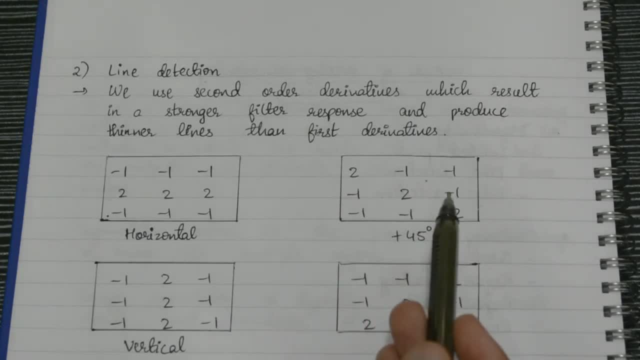 line plus 45 degrees, then we use this filter. okay, And for minus 45 degrees, we use this filter. So any given line, detection of any given line plus 45 degrees, then this and minus 45 degrees, then this. okay. So just note down all of these filters. okay, They are. 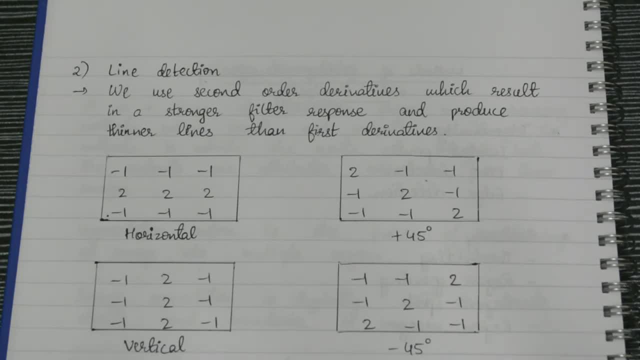 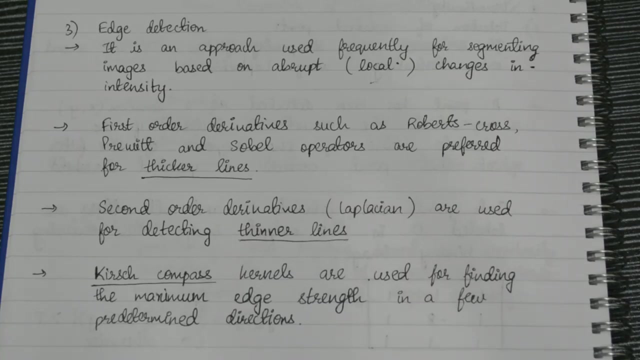 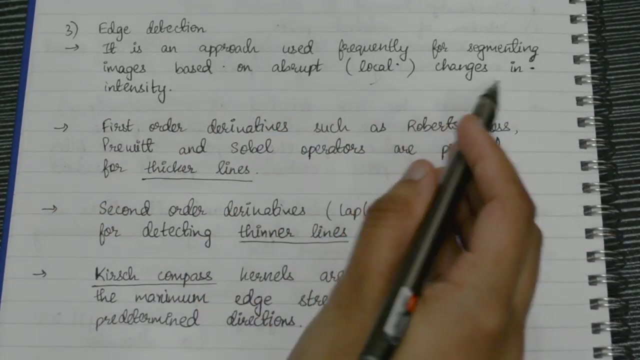 really important and they can be asked in the questions. So the standard procedure is the same, just that you have to apply all of these kernels on the images. okay, Only the kernels will change. Next we have edge detection. janji is this? So we have to use edge detection, And it is using lineшеf, So it is an approach. 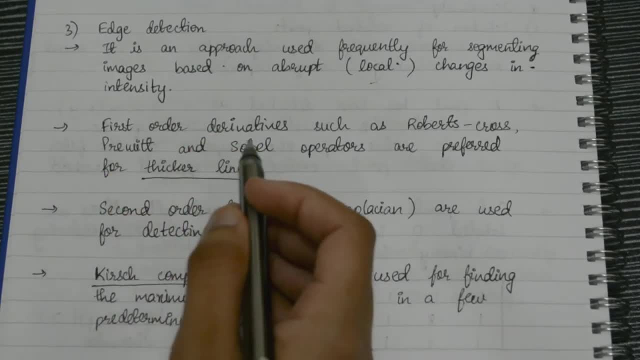 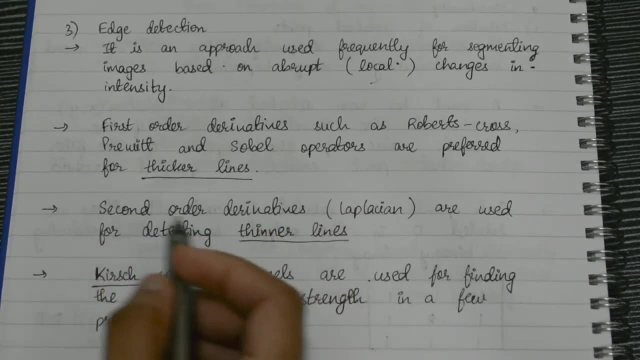 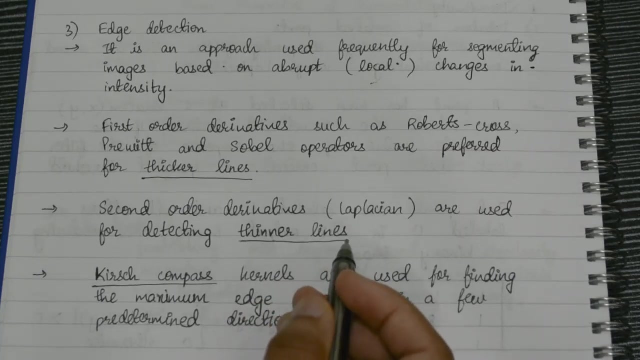 used frequently for segmenting images based on abrupt local changes in intensity. okay, The different types of operators used here are: first order derivative, such as rowboard, cross privet and Sobel operators are preferred for thicker lines, And second order derivative, such as laparation, are used for detecting thinner lines. 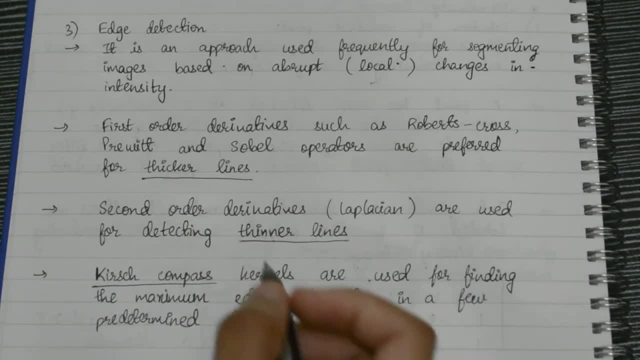 detect, then we use first order derivatives and for detection of thinner lines we use second order derivatives. so that's why most of the time second order derivatives are used, because they detect thinner lines. okay. but apart from these two, for edge detection there's the third kind of kernels. 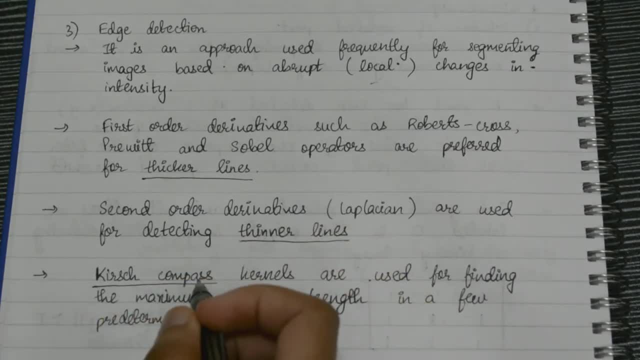 which are used, and those are known as krish compass kernels. okay, so these are used for finding the maximum edge strength in a few predetermined directions. okay, so these include additional directions and let's look at those kernels now. now, before moving ahead, i had made a video on 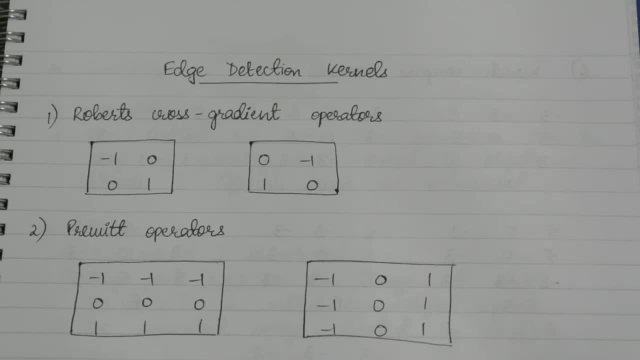 first order derivative filters, which involved robert cross, privet and sobel operators. so if you haven't watched that video, then kindly do so before watching this one, so that it will be clear to you how these mask are applied. okay, so now again we have the first order derivatives, which is, which is robert cross. 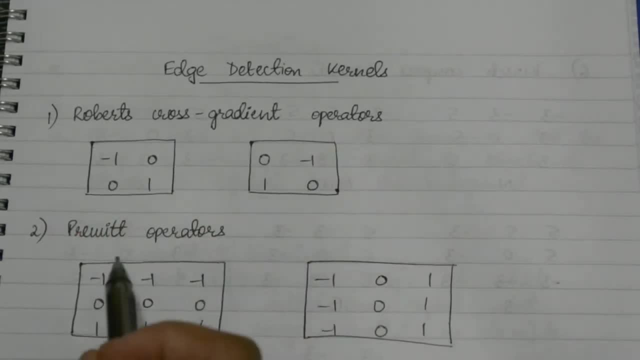 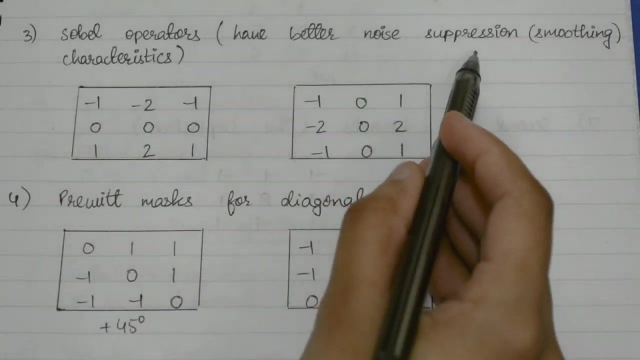 gradient operators- okay, so it is this. and then privet operators we have, which are three by three matrices, okay, so kindly note these down. then we have sobel operators, which have better noise suppression or smoothing characteristics. okay, so if these are applied, then we have the first order derivatives, which are the first order derivatives. 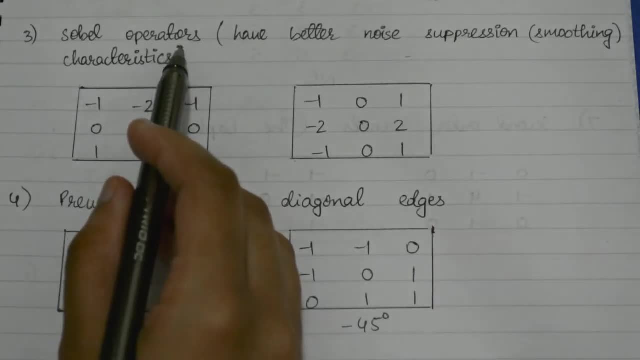 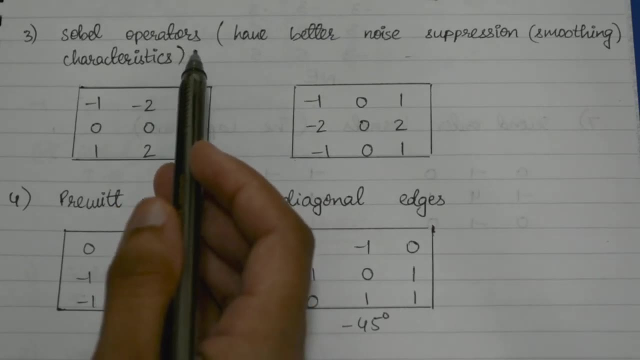 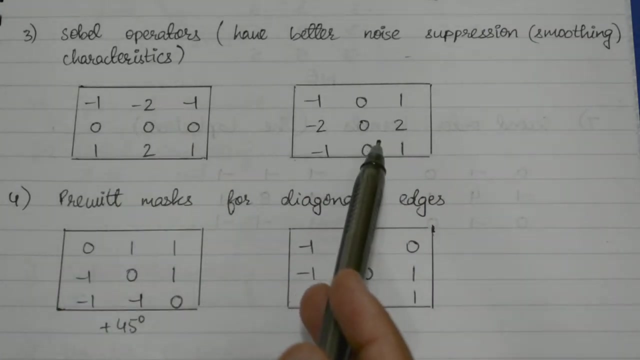 okay, so that is why these are considered better than privet operators or robert cross, because they have better noise suppression smoothing characteristics. okay, so these are the two filters here which come under sobel operators. and then we have privet mask for diagonal edges. okay, so for plus 45 degree angle, we have this one, and for minus 45 degrees we have this.